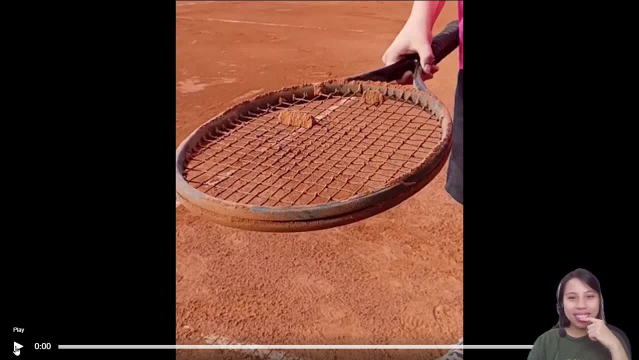 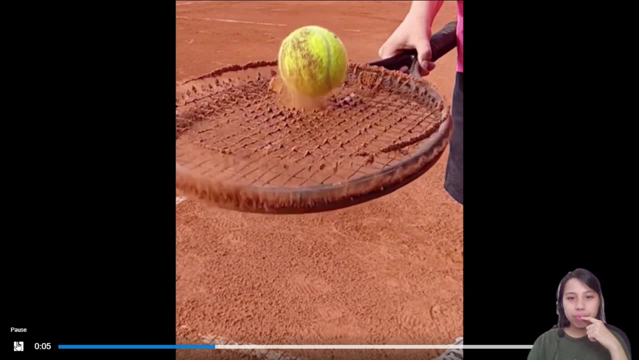 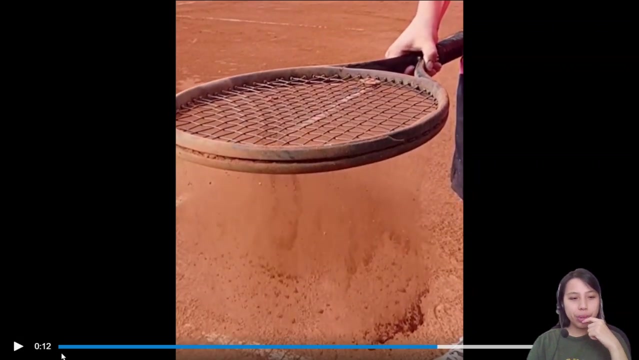 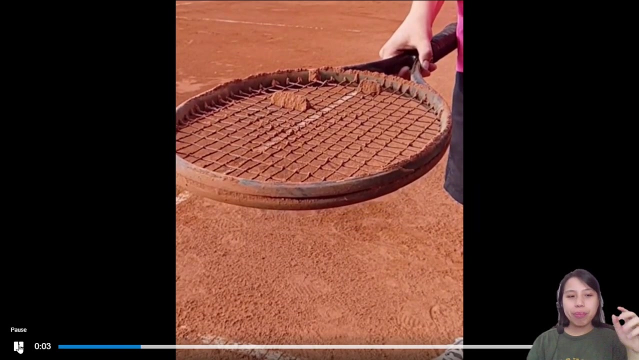 what happens to the dust on the tennis racket. Let's look and see In slow motion. Okay, if you didn't catch it, let me rewind to that spot and pause for you to see The dust, the racket. everything is pretty much chilling there. Suddenly, a tennis ball comes. 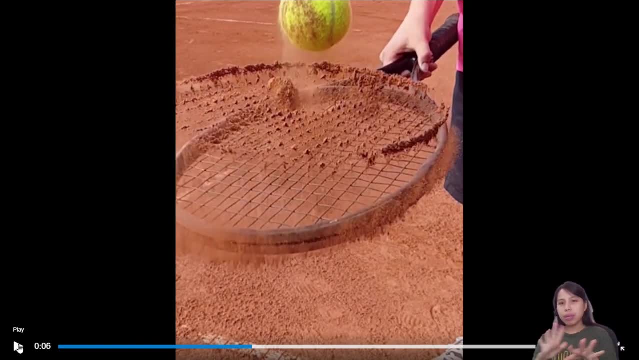 and knocks the racket away. Now, in this moment of time, something looks very strange. You see this shape of the racket in the form of the dust. Why the dust? It doesn't fall down straight away, leh? Why the dust want to chill there? That is the answer to the definition of what is mass. 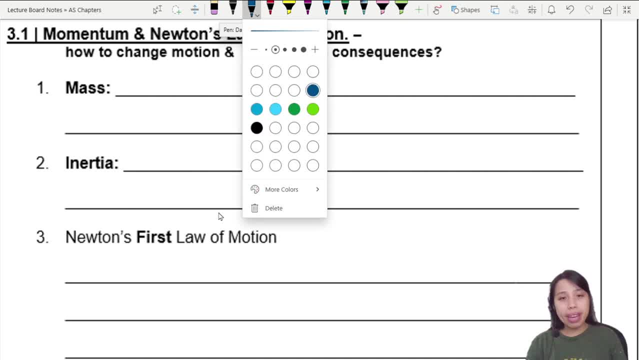 So in physics we come to this definition of mass that goes something like this: What is mass? ah, How heavy are you? 60 kg, Is that a mass Kind of? We kind of define this mass as the amount of matter, Or also- we can use this word- the amount of inertia. 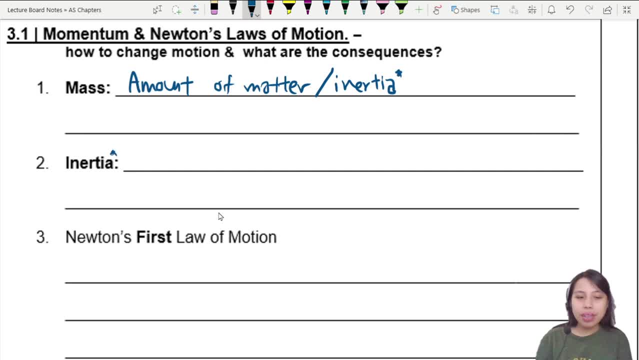 What is inertia? Inertia, there is a term we use as a tendency. Let me write that down: Tendency for something to maintain its motion. So how do we write the explanation? It's a tendency. to maintain its state of rest Means not moving. 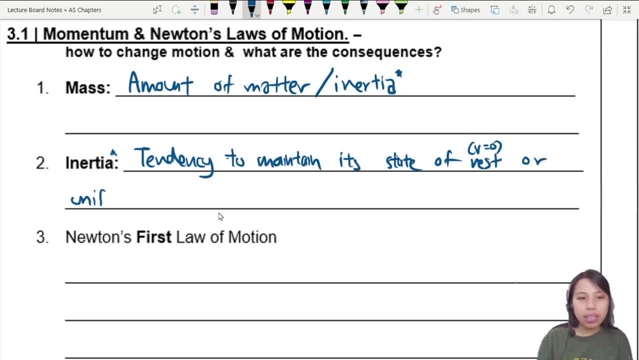 Okay. Or Uniform motion in a straight line. Motion in a straight line, Which means uniform motion in a straight line, also known as the velocity, which is a vector, Cannot change direction. ah, Is constant, Okay. So in other words, it's like a resistance to motion, To change in motion. 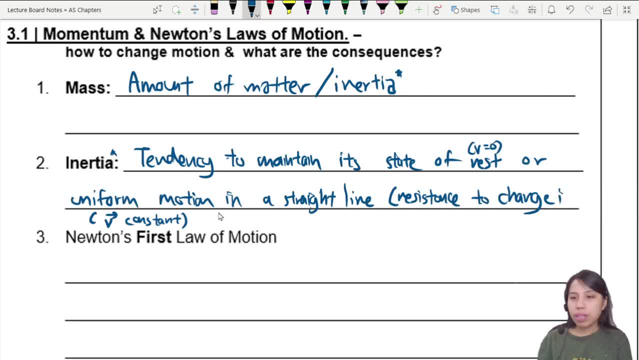 Resistance to Change In motion. Aiya, no space. ah, right, here lah. Let's look at that carefully again. So you got mass means you got inertia. Got inertia means you don't want to change motion. Very stubborn, In other words, if you are very heavy, you keep moving forever and ever. 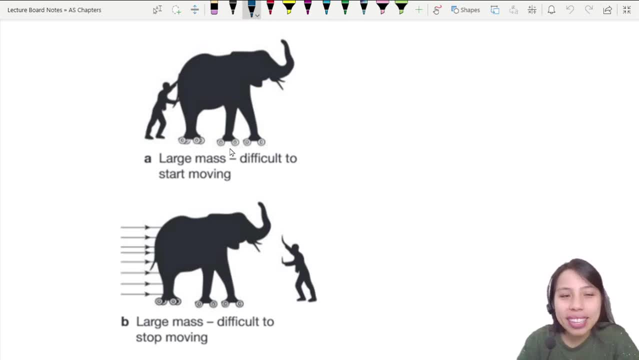 For example, a big, big, big, big elephant. Let's say, this elephant is I don't know how. actually I don't know how heavy this elephant. Maybe Google and see lah, but I just want to write 100 kg. Maybe Google and see lah, but I just want to write 100 kg. 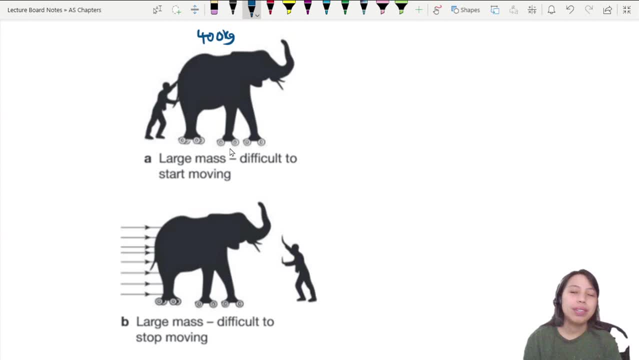 okay, maybe 400 kg. that's really heavy, never mind 400 kg. and then you, your elephant is at first at rest. then this poor guy wants to push the elephant to get it to move. is it gonna be a tough job? yes, very hard to push, like very hard to push. the elephant does not want to move. but if the elephant 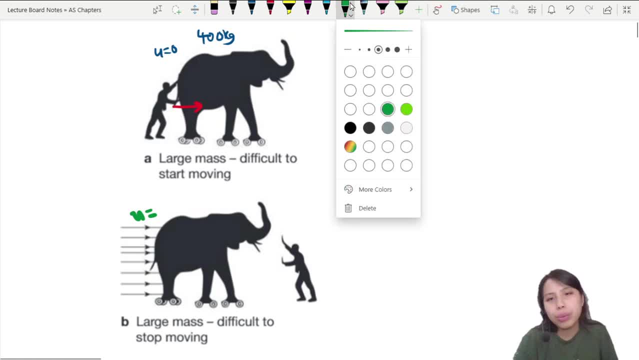 is already moving at a super fast speed. why would the elephant be on roller coasters? i don't know, maybe moving at 5 um 15 meters per second, which is really fast, and then the poor man say stop, stop, stop, stop moving. it's gonna be very hard for the elephant to stop because 400 kg, so much inertia. 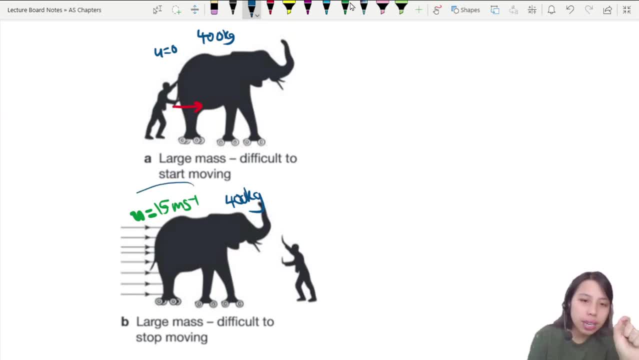 it cannot stop. so you see, once this elephant is moving, if we assume there is no friction, no friction, this object will keep moving forever and ever and ever until somebody say stop, stop, either friction or some other force. it's also kind of similar. okay, imagine this. is you lying? 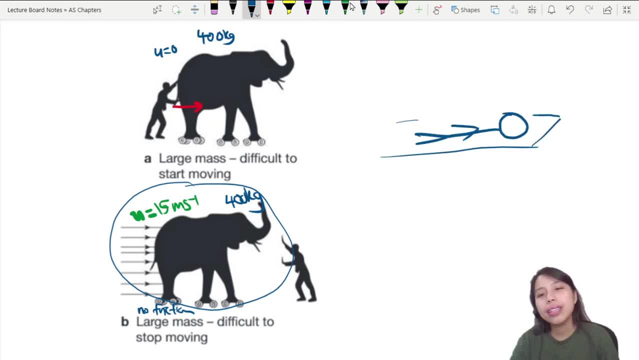 on the bed. wow, very nice. ah, lie on the bed. got morning class, got something i are very hard to to start moving, right, because you have mass, you have inertia. what's your inertia? 60 kg, 50 kg, 80 kg- very hard to get out of bed, okay, but once you start moving, already, or very hard to stop running. 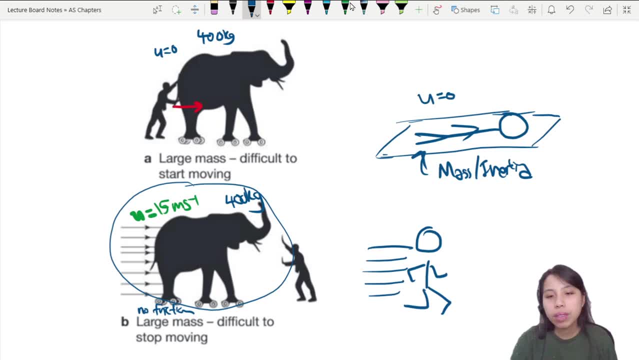 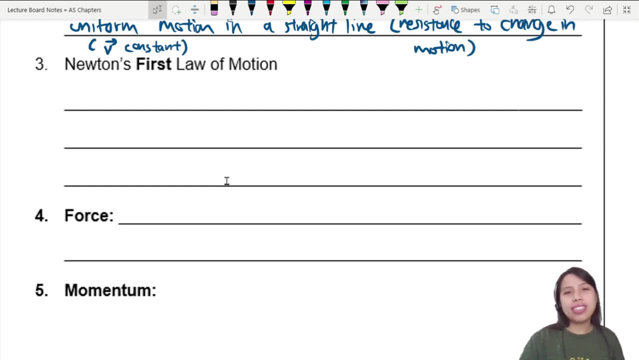 for example, let's say i'm running super, super fast, it's hard to stop because of inertia. so mr newton sat down he stared at all this elephant and things and he said: let's make this official, let's make a law, the first law of motion. so newton's first law of motion. so you should know the definition: a body or any object. 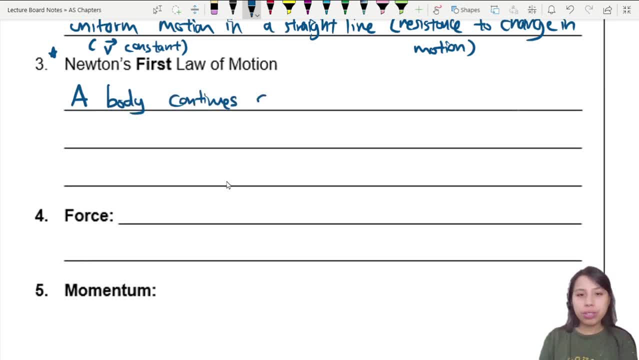 will continue, or continues at rest, or continue at constant velocity, unless something stopped the object. so we say unless acted on by a resultant. this can be many forces, but we just say overall. resultant means add together all the forces, so resultant or external force. there we go. okay. so imagine i take a ball, i roll it along a horizontal surface, if i assume there's no friction. 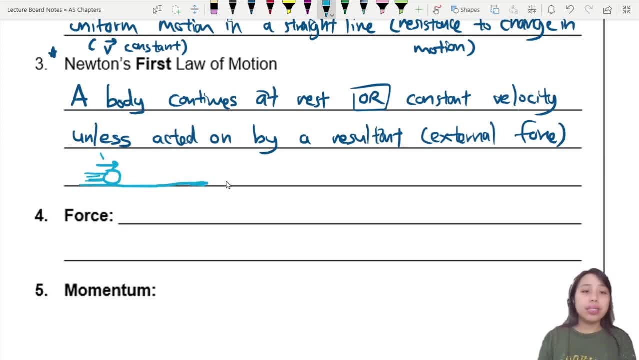 this ball should continue forever and ever and ever at the same velocity until it hit a wall or hit some some mud. so this one, uh, the key idea is either at rest or constant velocity. all is based on the same idea: that there is no change in velocity. then keep going. 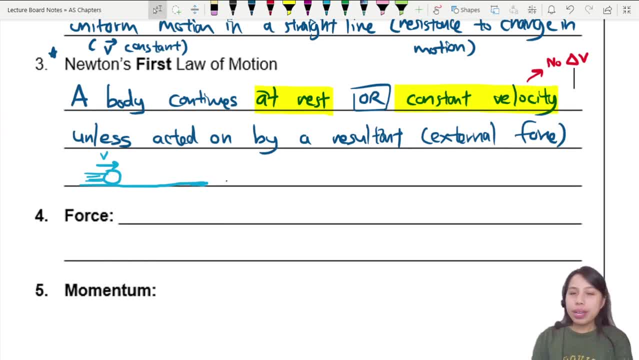 if you're at rest, you chill there. if you're moving, keep moving. by the way, a side definition of force which is down here, it's a, it's an informal one, but in case you are finding it hard to understand what is force, you can explain it as kind of the push and pull. 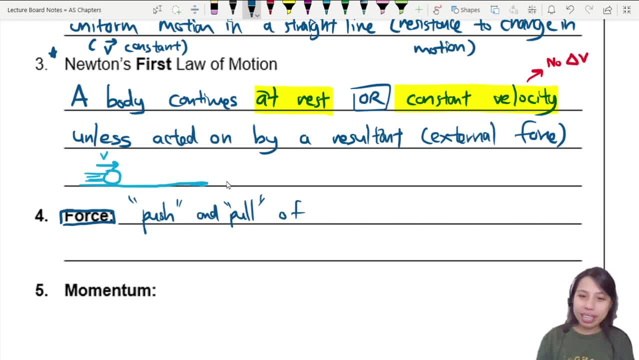 of an object, of an object. what does the force do? it causes it to change. it causes it to change, Change velocity or change shape. So once again note: this is an informal definition of force. Later, in another video, you will learn the formal A-level definition of force. 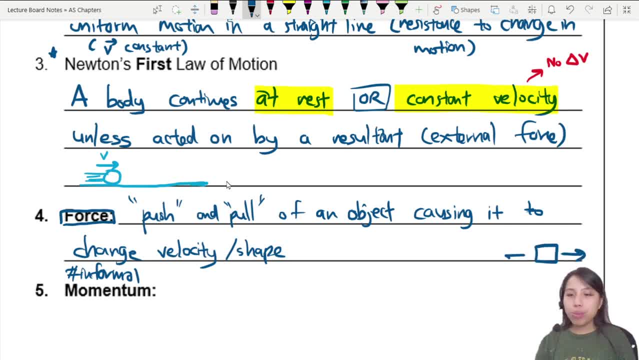 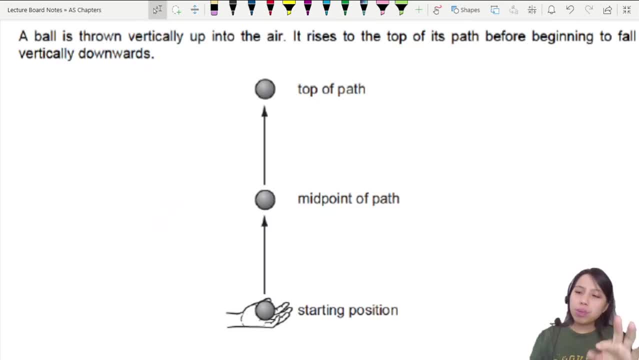 So imagine we've got a ball here, You pull this way, you pull that way, maybe you'll squash like that. Then you'll change shape, start moving and things like that. Okay, now, before we move on, let's pause and exercise our brain a bit. 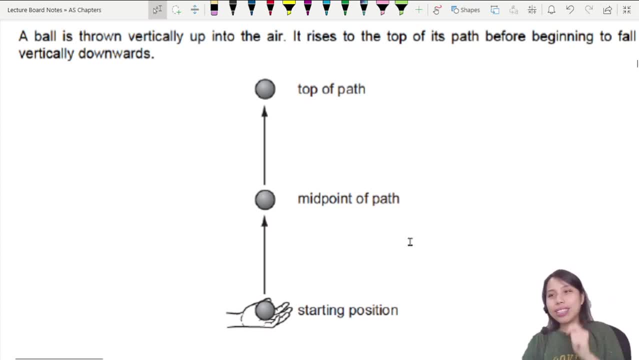 Here is a picture I took from a bus. here I'm going to change it, I'm going to ask our own question. So here you have a ball thrown vertically up into the air. We've seen this many times in kinematics. So the ball goes up to the top before it comes down. 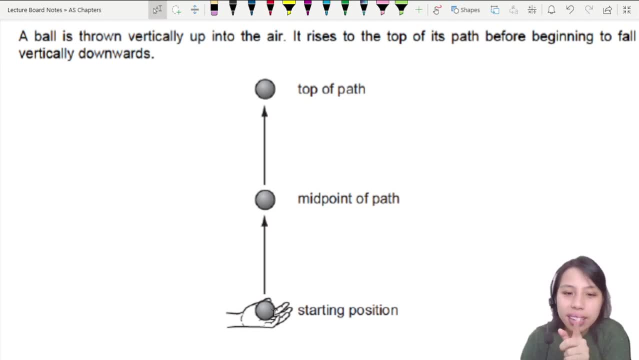 Now let me ask you: at which point is there a force from the hand on the ball? Or I should say: actually this ball can go up. What keeps it going up? So I'm going to write that out: What keeps it going up? 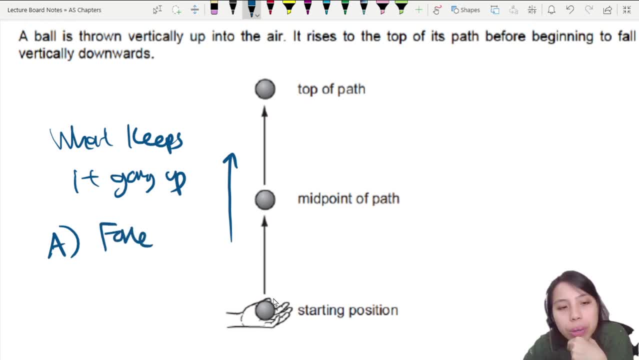 Choice A: force on the ball. Choice B: something else. I don't know. What do you think? Pause this video if you need to think a little bit longer. What keeps the ball going up? Why it can go up one. 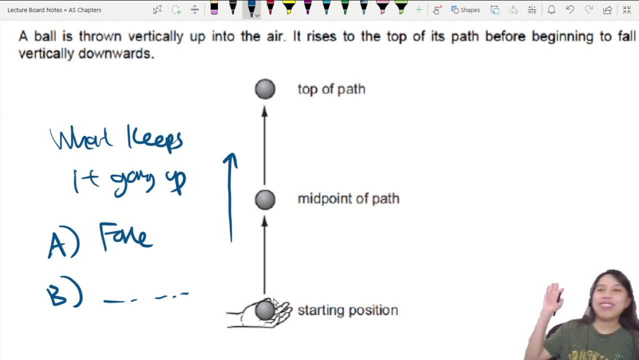 Now, if you thought about this carefully, in kinematics, this question is like: I understand now, But, but, but wait. So actually it is not a force that keeps the ball going up, It's something else. The answer, if there were anything, would be inertia. 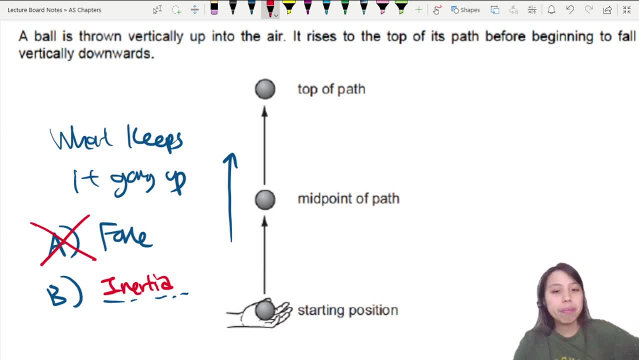 Huh, Inertia, Got equation one. ah, No equation, It's just a concept. The moment when the ball is in contact with the hand, that moment down there only got force from the hand. Give you an initial push, Okay. 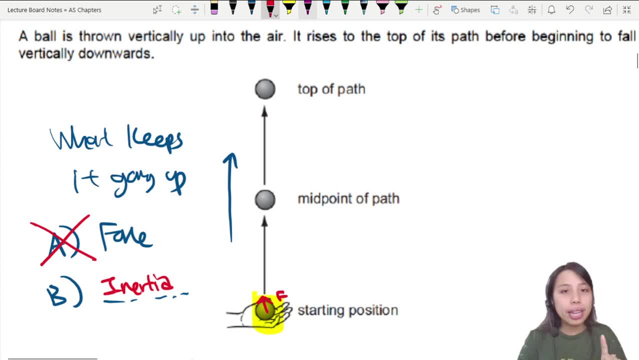 Then, once the ball is in the air, not touching the hand anymore, The ball is in the air, not touching the hand anymore. The ball is in the air, not touching the hand anymore. The ball is by itself already Only got one force pulling it down. 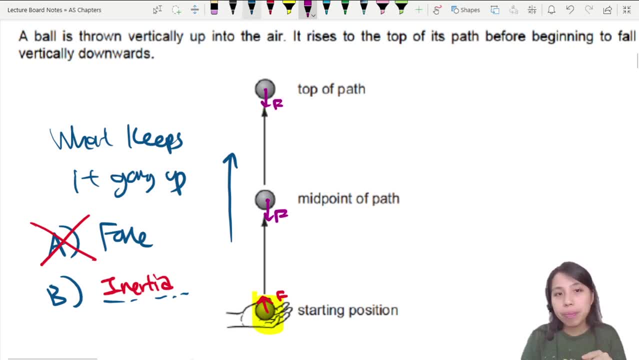 Nani, You see, this force is pulling it down, not pushing it up. So what keeps it going up? Inertia Until, eventually, you run out of energy and then no more final energy already. Okay, So remember, ah, what keeps the ball going up? 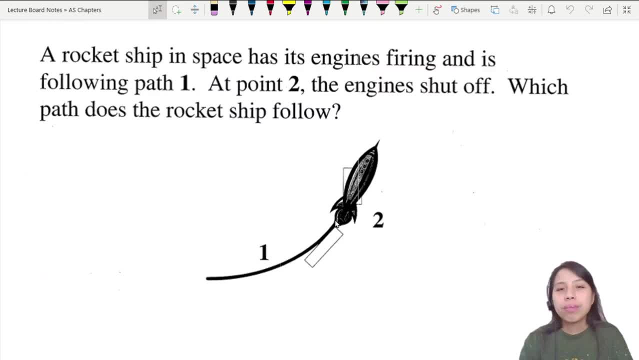 Inertia, not force. So likewise if you have a rocket ship in space that is firing and travelling in this nice curvy path, So likewise if you have a rocket ship in space that is firing and travelling in this nice curvy path. 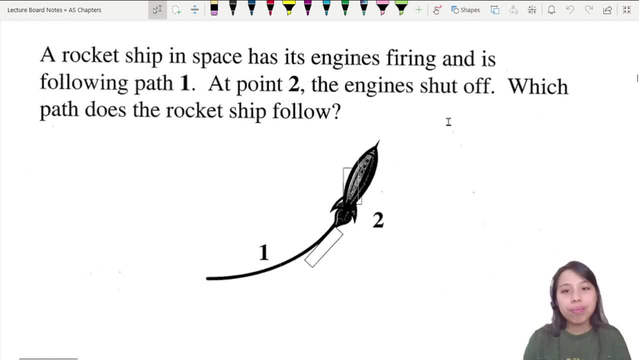 Travelling, travelling. Suddenly at point two, the engines shut off. What path does a rocket ship follow? I'm going to assume there's no other forces in this universe, So how would the rocket ship travel After that go? continue like this? 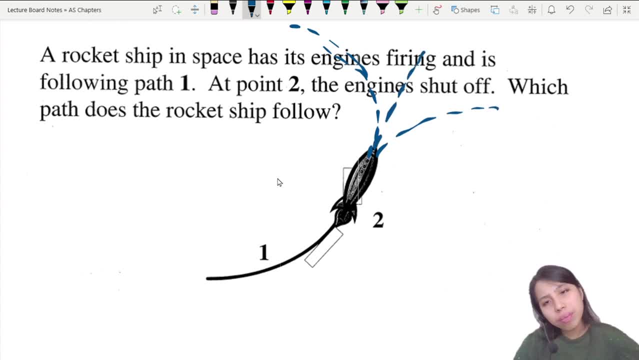 Or go like this, Or go straight line. How will we know? Think of inertia. Oh, an object will keep moving at a constant velocity. So means whatever. At point two: ah, there's no more force already. So if there are no forces acting on the object, it will just keep moving in a straight line. 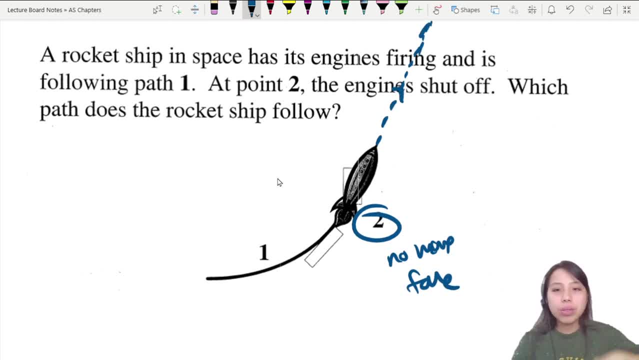 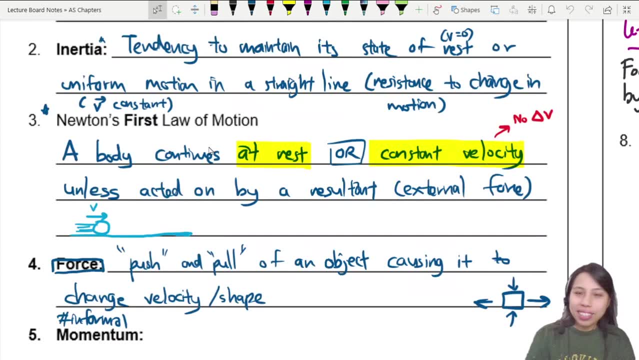 Until it hits something or another force acts on it. Okay, so that is the path I'm going to go, where it is, on a constant velocity, including the direction. Now, a lot of students keep asking me But but, but, Miss, isn't there an equation for inertia, or something like that? 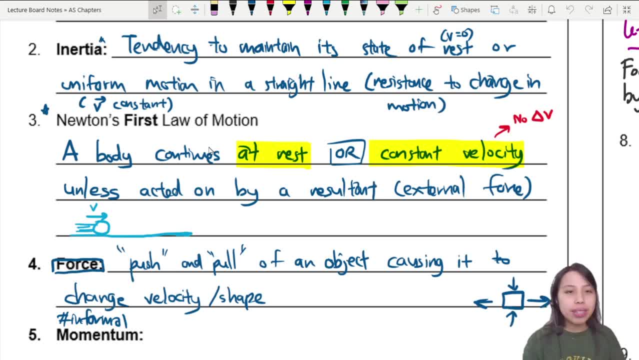 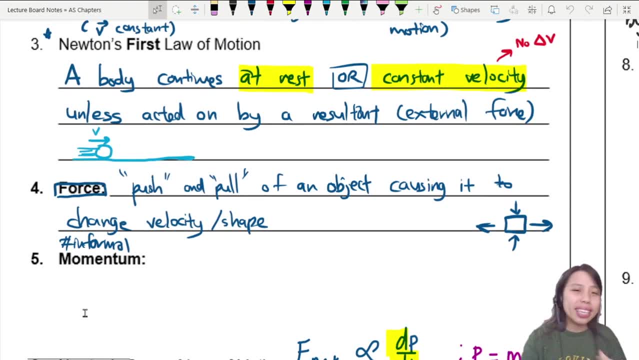 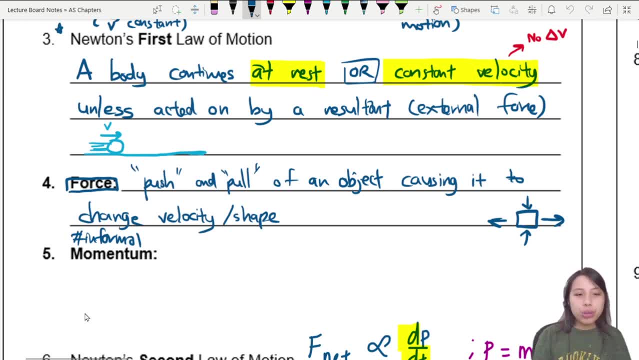 Momentum. you see down there is. we use the symbol P for momentum like: oh, I don't know why we choose P, But okay, For momentum. we take mass times, velocity of an object. And don't forget, momentum is a vector, Velocity is still a vector. 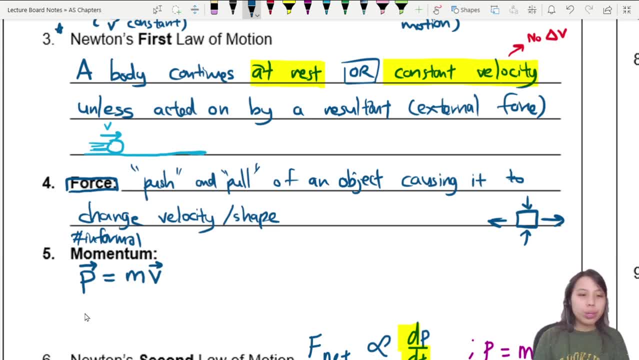 So direction matters. So if you want to define what momentum is, if you're interested, go on YouTube to find out more about that Momentum is. we just talked about the equation. We say this is the product of mass and motion. It's kind of like a quantity of motion. 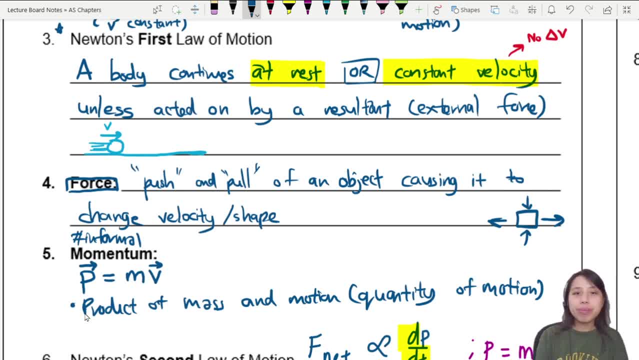 Inertia. How much Calculate momentum? Calculate momentum Save. Give us a number that we can actually use. So this one equation, you will use it a lot in A-levels. Is there a unit for it? Yes, Mass times, velocity. 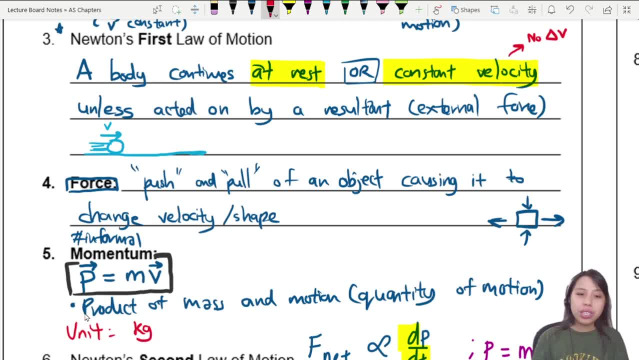 So the unit will be mass kg times. velocity ms negative 1.. You will see another unit for this later, but I'm going to write it down. That unit will be force times second. That's an interesting one, But we only know where that comes from when we look at Newton's second law down there. 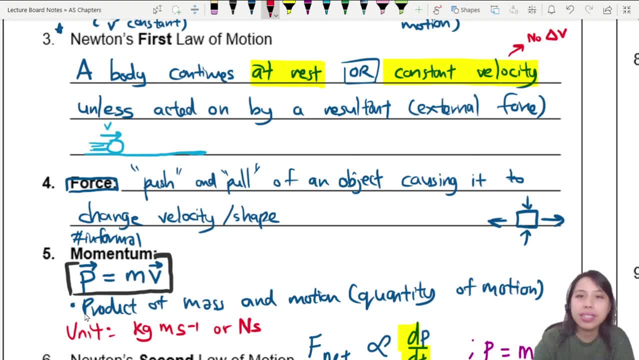 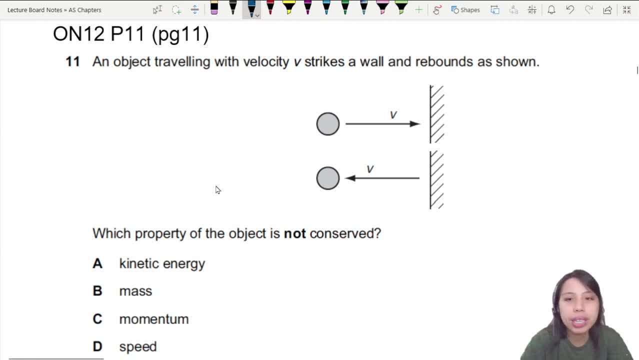 See it's picking up already. Okay, so momentum. How do we better understand this? Here we have an object travelling with a velocity v, hit the wall and bounce back- Ping-pong-pong- Okay, kind of like a collision here. 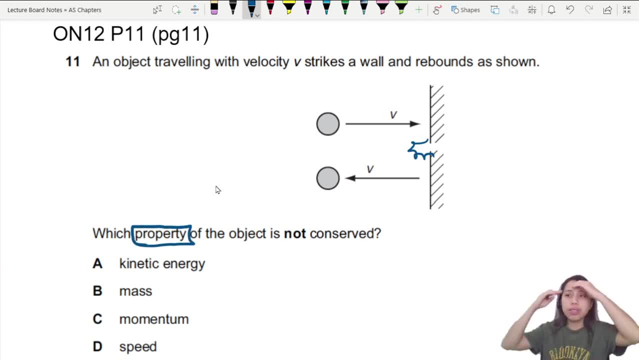 Which property of the object is not conserved. What does conserved mean? Conserved is a word you will see a lot. It kind of means like same before and after, Didn't change After something happened. Well, here the something happened is the collision that happens in a moment in time. 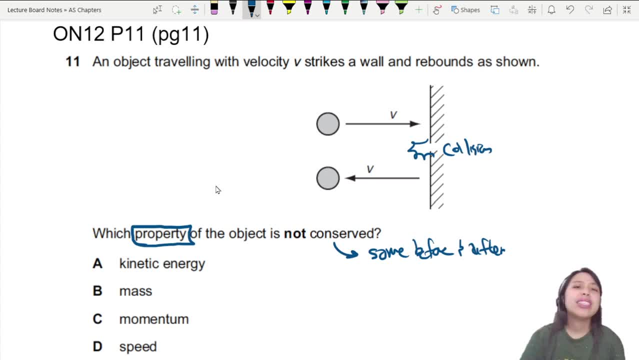 Okay, But it's not the same. Let's look carefully at what are the choices. First choice is kinetic energy. What's kinetic energy? again, Kinetic energy we know as half mv squared. So you see the speed of the ball. V. 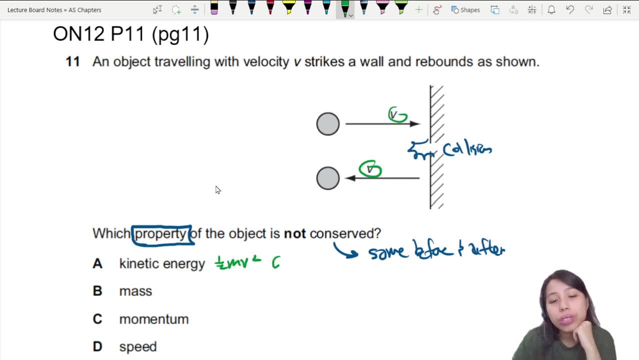 Then after that collision, also v, Then same, So same, no change. So it's conserved. Okay, we want the not conserved one right? So this is not the answer. Let's look at mass. Did the mass of the ball change? 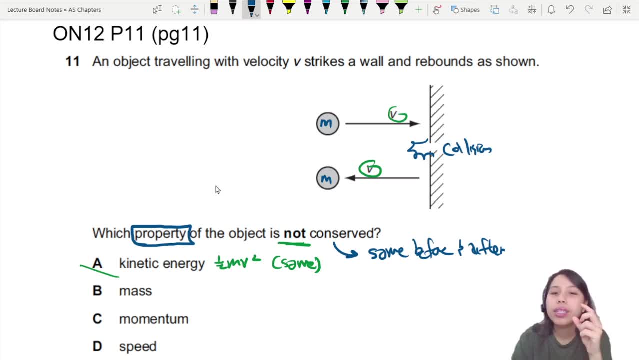 Here is mass. Here is mass, No more. They didn't say So. did the ball break in half, Explode, Become dust, Nope, Okay. so mass is the same, Or the mass is conserved. Momentum and speed. 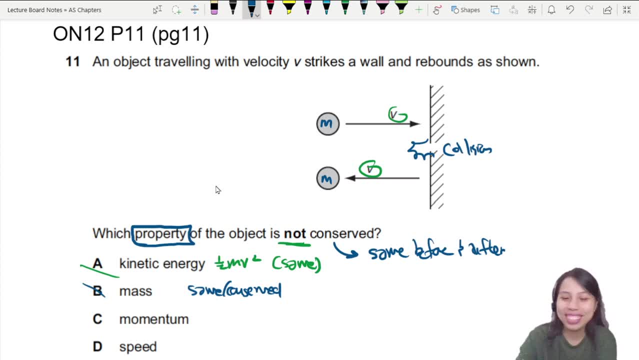 The last two choices, Which one is conserved? I would say that speed is conserved. Same Speed is conserved because it is v At first, initial, it is v After collision, final it's still v, So speed is conserved. 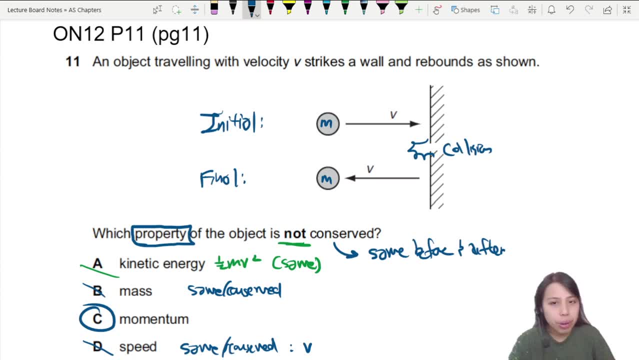 That means momentum is the answer. But why is momentum not conserved? Because if we try to calculate the momentum of this ball or collision happening here, the direction actually matters. So in the beginning, this ball, before it hits the wall, the momentum of mass is mass times velocity. 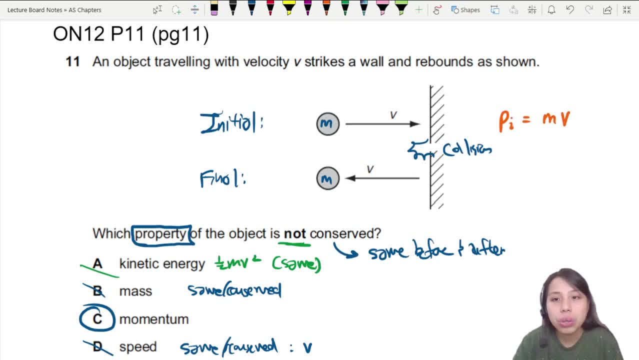 But wait, velocity got direction, So we need to choose a direction. Okay, we see, everything to move to the right is positive. Anything that moves to the left is negative. You define this, So this is positive, v Okay, good.